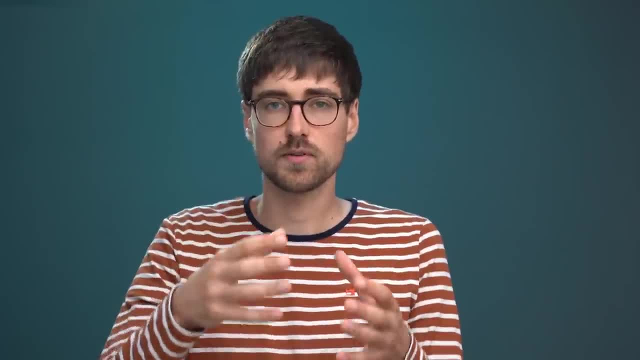 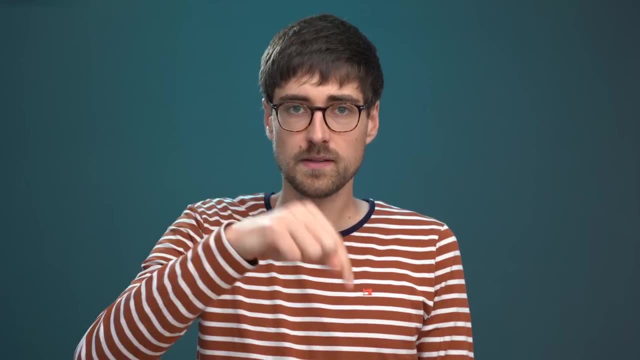 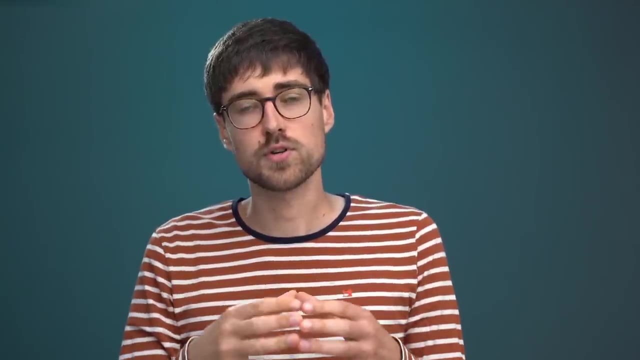 random location, then the probability for this marble to end up in one of the bowls is proportional to the bowl's cross-section area. And if we repeat this process over and over again, then also the number of marbles ending up in this bowl will be proportional to the bowl's. 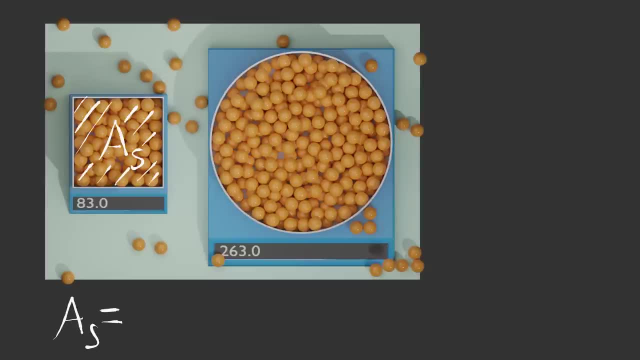 cross-section area. The area of the square bowl in this example is its edge length, a squared, And the area of the circular bowl is pi times a squared. And that's how we get pi as the fraction of the two areas and consequently as the fraction of. 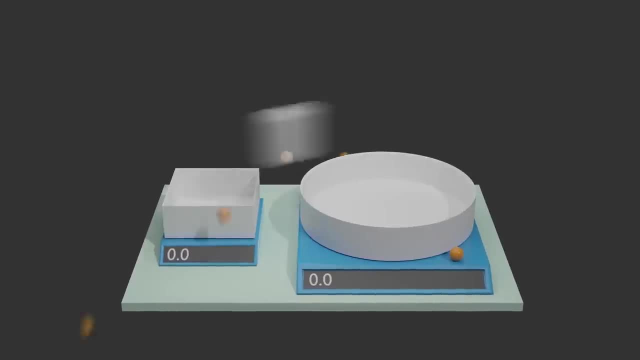 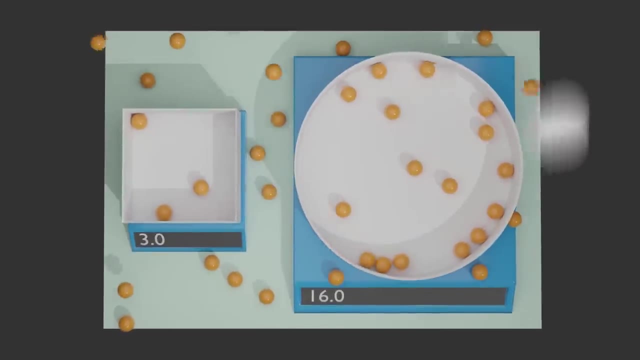 marbles in each bowl. So in this example of a Monte Carlo simulation, we essentially determine an area by taking random samples. With each random sample we probe whether this specific location is inside or outside of some area And by taking random samples we determine whether this specific 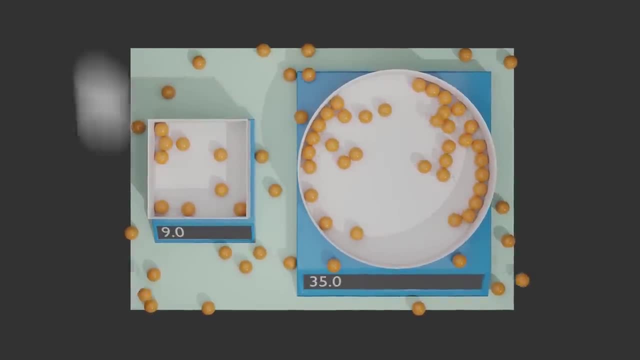 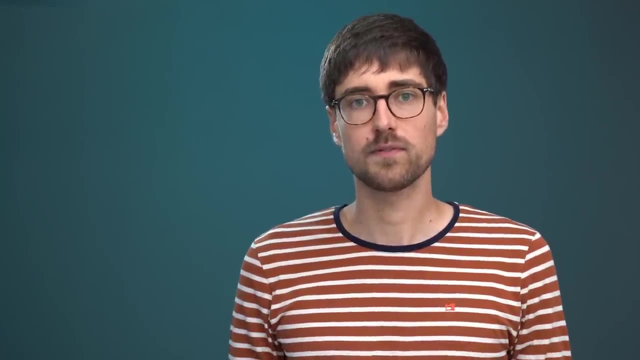 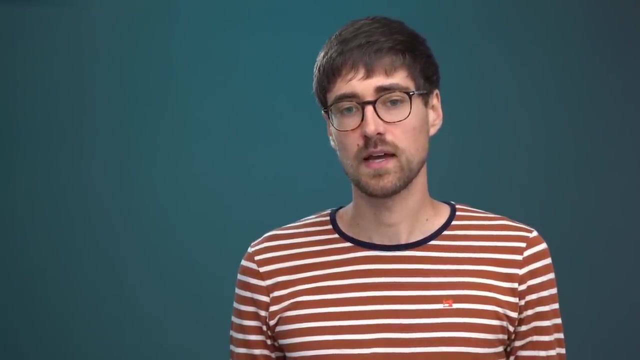 location is inside or outside of some area And by taking enough samples we get a good idea of how big an area is. This idea of obtaining random samples is probably quite familiar to you if you think about how real-world studies are designed. Let's say we wanted to find out the average height. 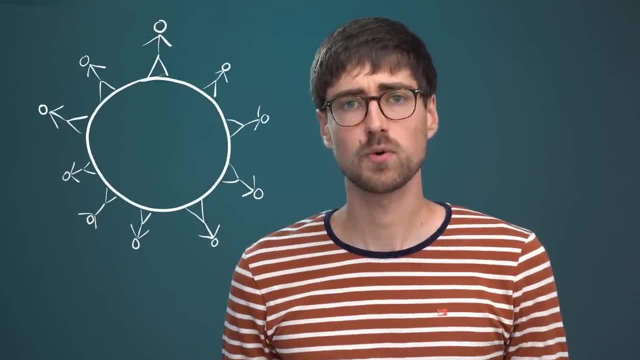 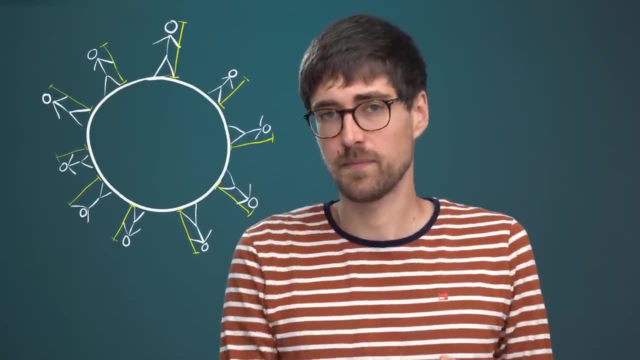 of all people worldwide, Then in principle we would need to measure the height of each person worldwide and then take the average to get an accurate result. But of course we can't go out and measure the height of billions of people. So what can we do? Well, 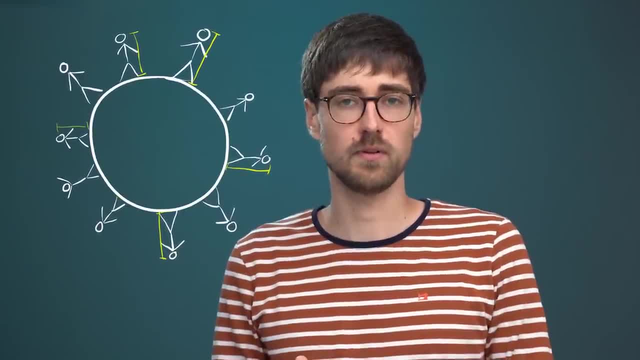 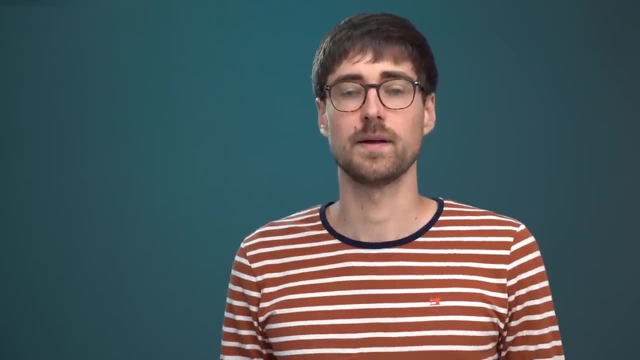 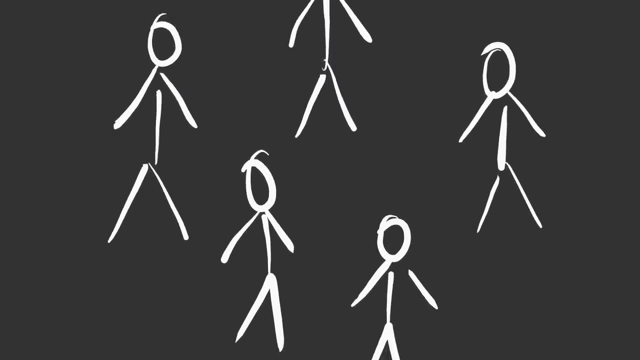 we can measure the height of some smaller group of people and hope that their average height is a good estimate for the average height of all people worldwide, But there are two things that we need to consider. Firstly, the selection of the group of people needs to be unbiased. 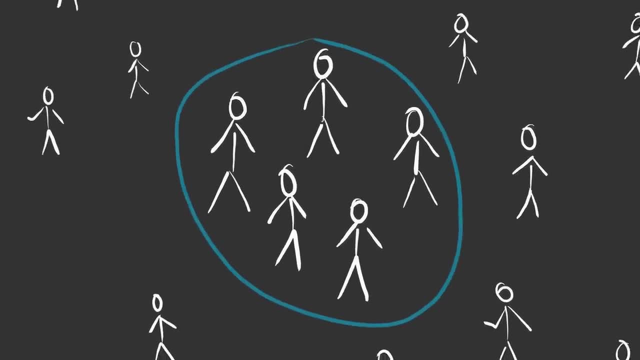 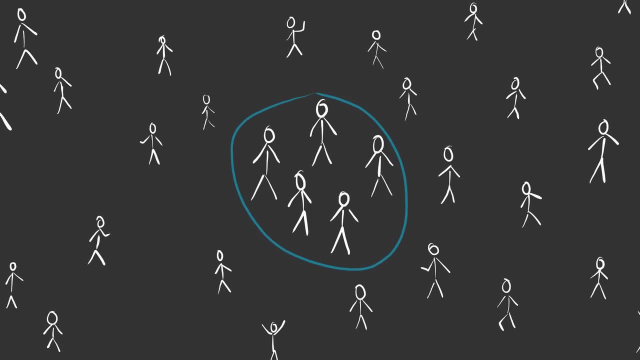 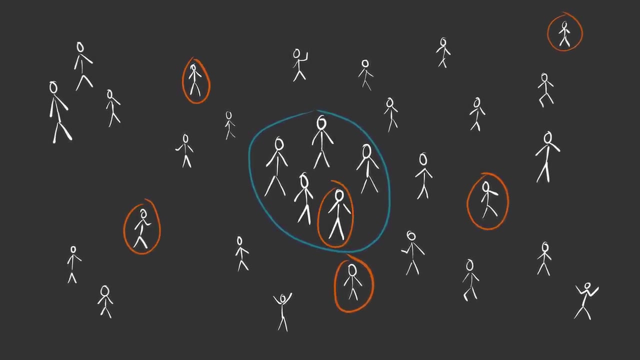 We can't just measure the height of the next five people we meet, as we might live in an area with especially tall or short people. A better way to get an unbiased sample group would be to randomly select people worldwide. Randomness helps us to make an unbiased selection And 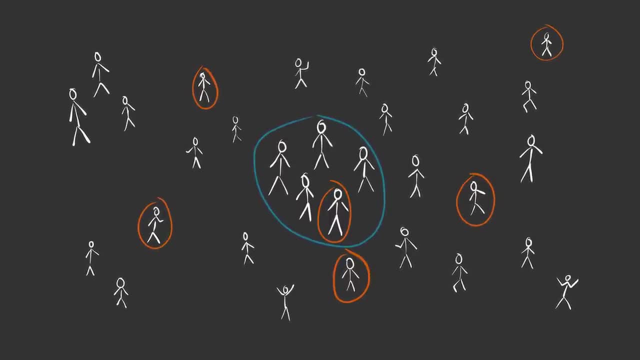 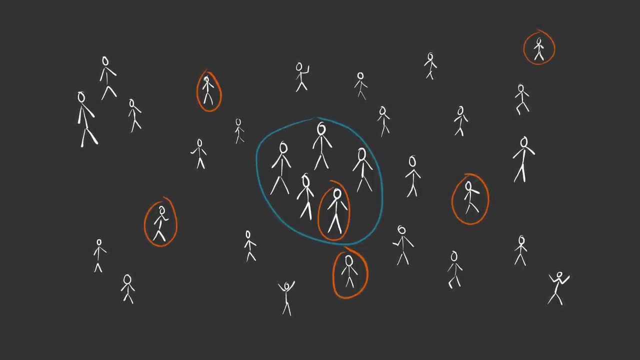 secondly, the group of measured people must not be too small. If we only measure the height of, let's say, five people, we might have just coincidentally picked five taller or shorter people And we can be more and more confident about the average height of all people And we 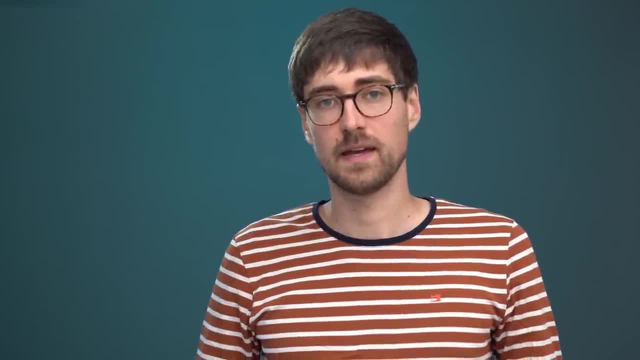 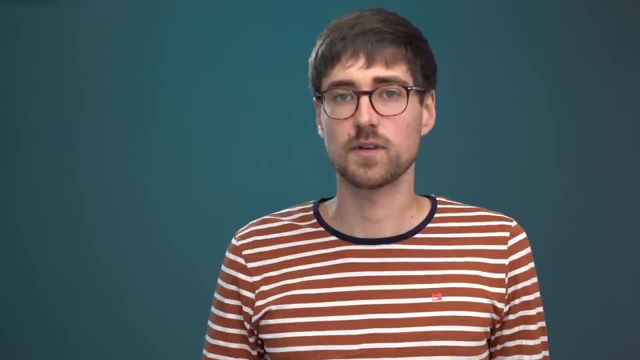 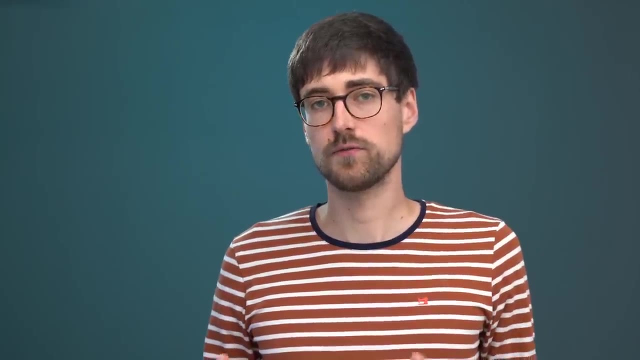 the average height, the more people we measure. In probability theory, this is called the law of large numbers, which essentially states that an average tends to come closer to its expected value the more samples we have, And the exact same is also true for Monte Carlo simulations. 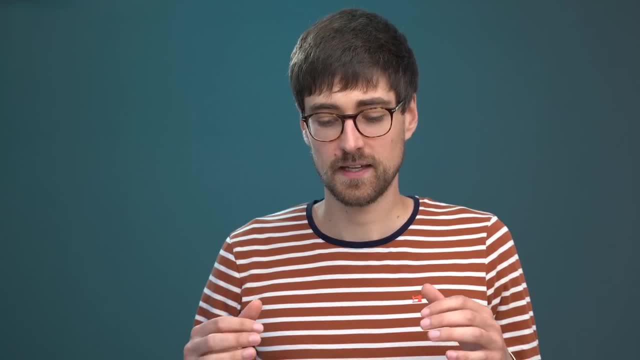 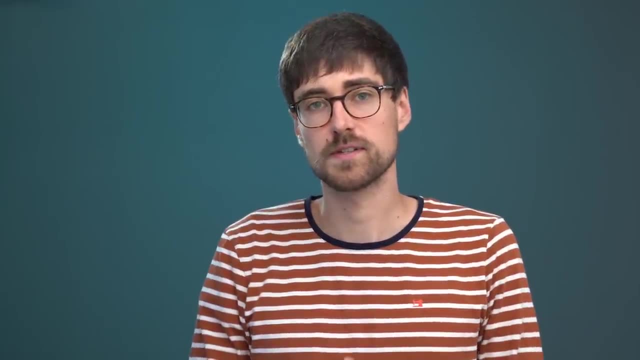 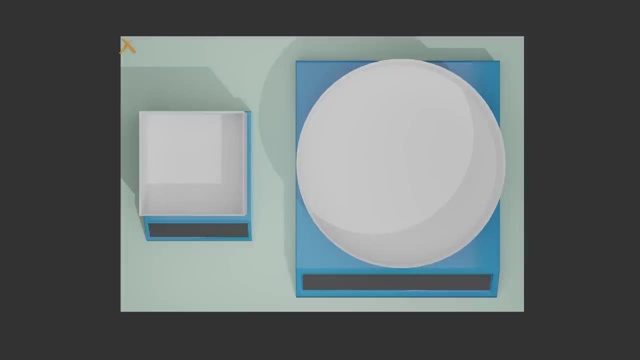 The core idea of a Monte Carlo simulation is that we can get an unbiased representative group of samples from some large ocean of possibilities if we allow the simulation to evolve randomly. In the marble dropping example, in principle we would need to test for every possible location. 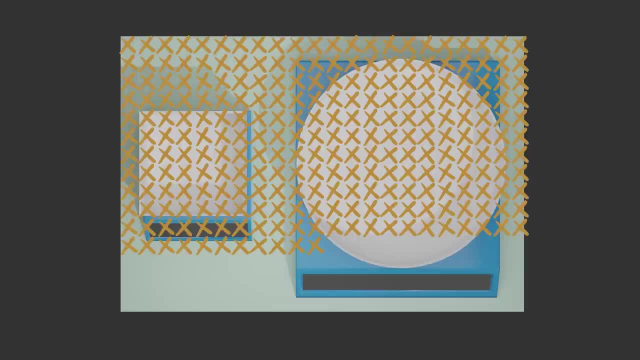 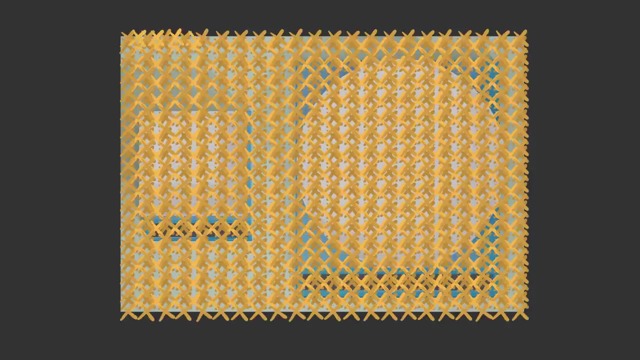 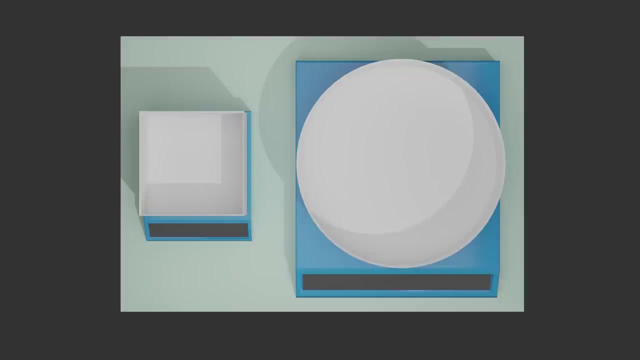 whether a marble ends up inside or outside the bowl to determine the bowl's cross-section area, precisely Just like we, in principle, would need to measure the height of each person worldwide to determine the average height accurately, And instead we can rely on randomly selected samples. 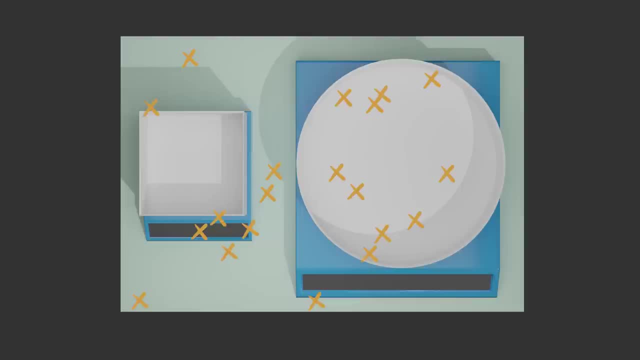 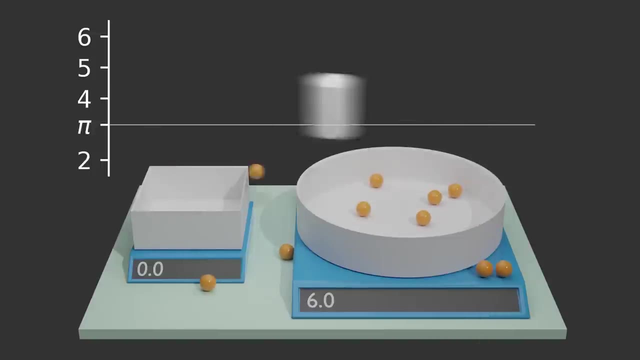 And according to the law of large numbers, we can be more and more confident about the result the more samples we take. We can see this if we plot the fraction of marbles in both bowls over time. Initially the value is fluctuating heavily, but with more and more samples generated by 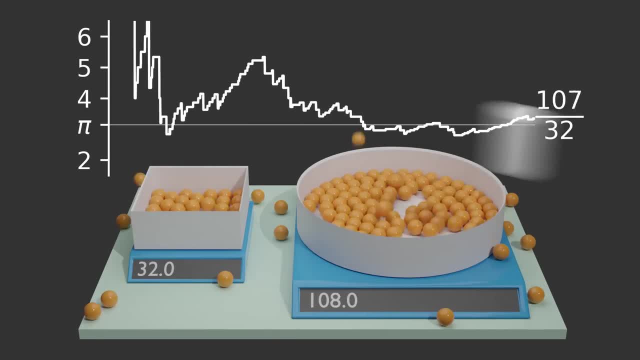 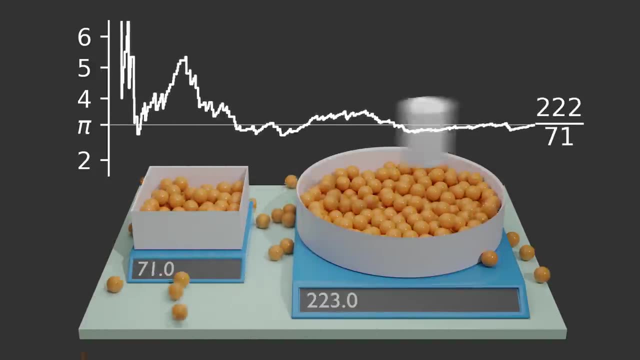 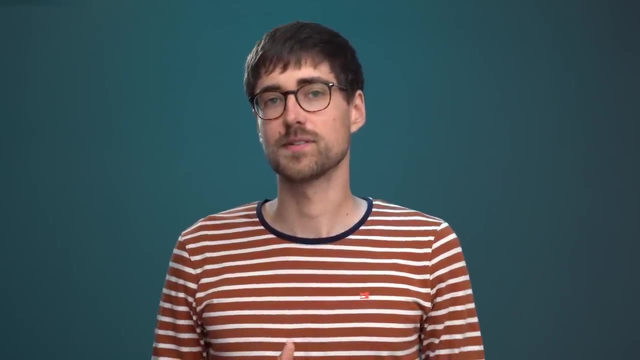 the randomly evolving simulation, the fluctuations become smaller and smaller And we can see that the fraction approaches the expected value, pi. Now I hope that using a Monte Carlo simulation to determine pi was an illustrative example, but it's certainly not really relevant. 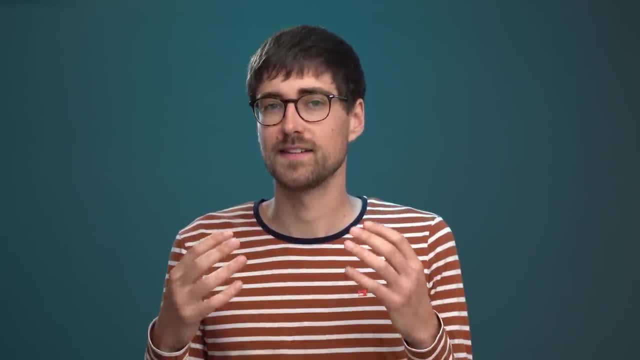 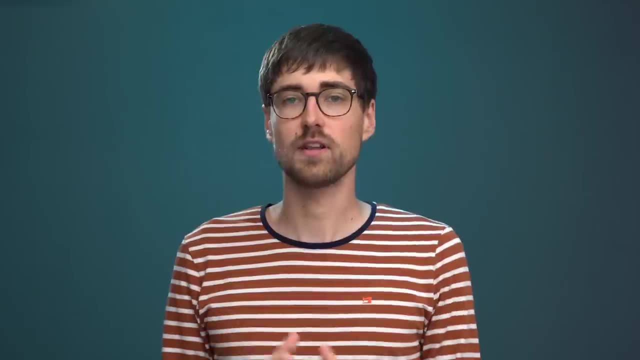 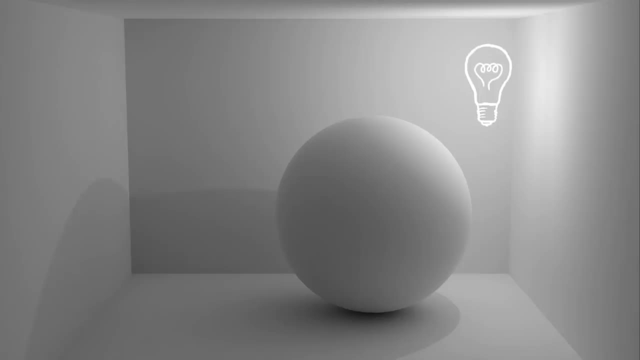 But actually this animation of dropping marbles has a second example of a Monte Carlo simulation somewhat hidden in it. so let's take a look at this hidden, more relevant example of a Monte Carlo simulation in the last part of this video. Rendering such animations, or the simpler example scene, is all about simulating the. 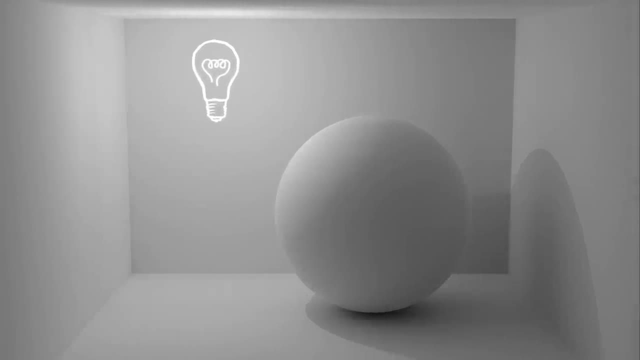 flow of light. To get an accurate image, you need to find out how much light hits different areas of the scene, And this is not an easy task if you consider that a few surfaces can scatter light in virtually any direction. So let's say we want to find out how much light hits this market. 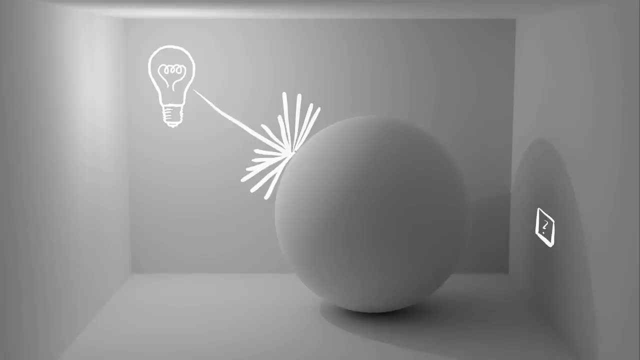 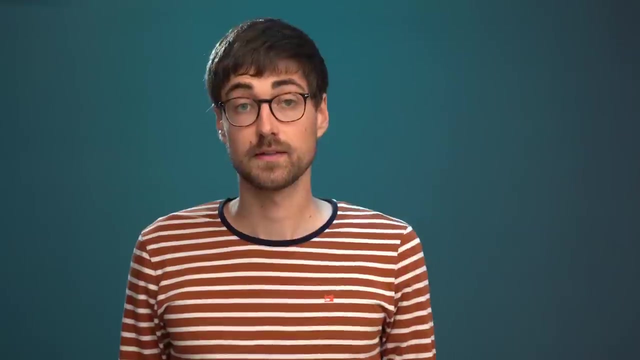 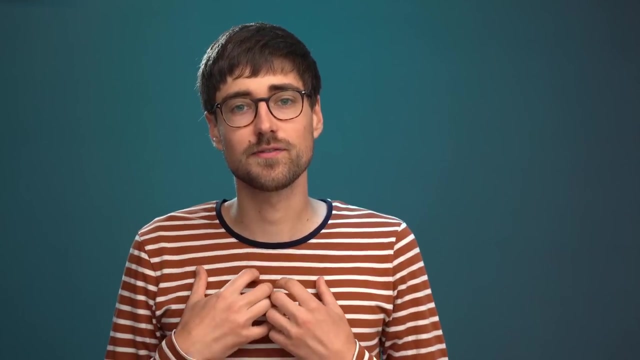 Then, in principle, we would need to evaluate all possible light paths to find out which fraction of them ends up in the marked area. Now, clearly, it's impossible to follow all the possible light paths. So what can we do if we can't follow all possible paths? 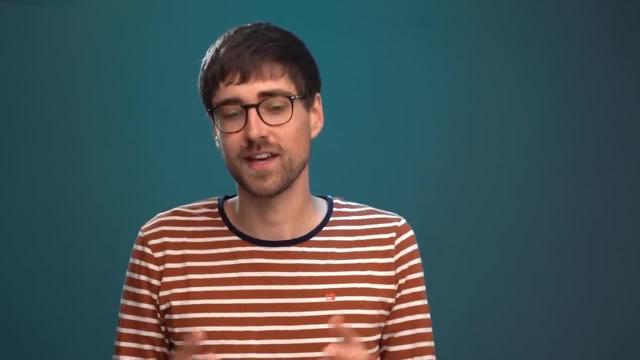 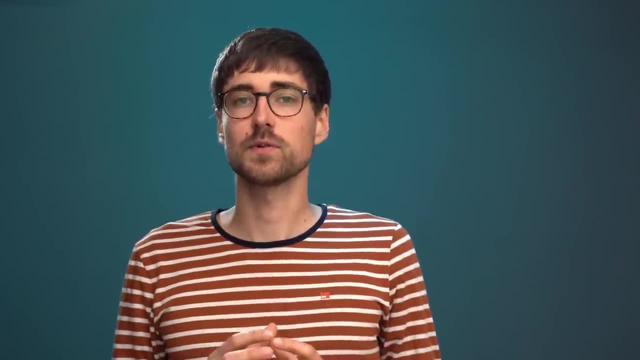 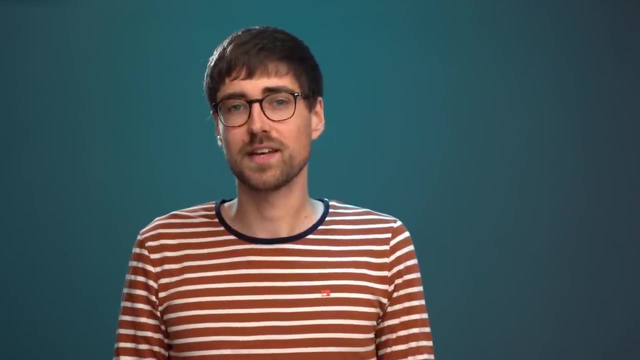 Well, I hope that after watching the video to this point, the answer is quite obvious. If we can't simulate all possible light paths, Then the best we can do is to simulate a representative group of sample paths. And what is a good way to get an unbiased representative group of samples? 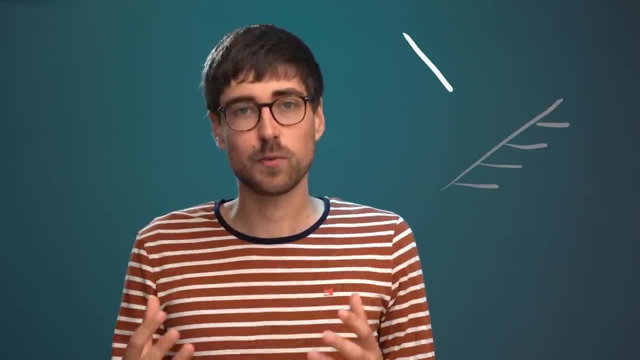 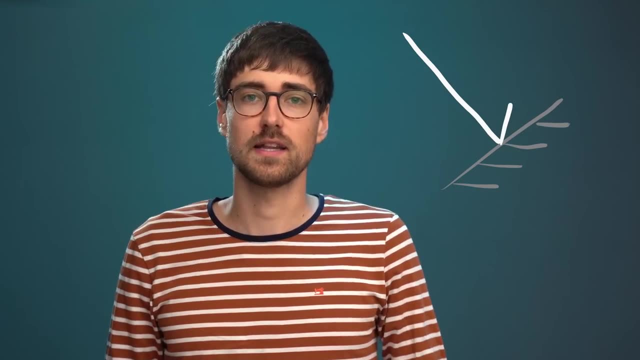 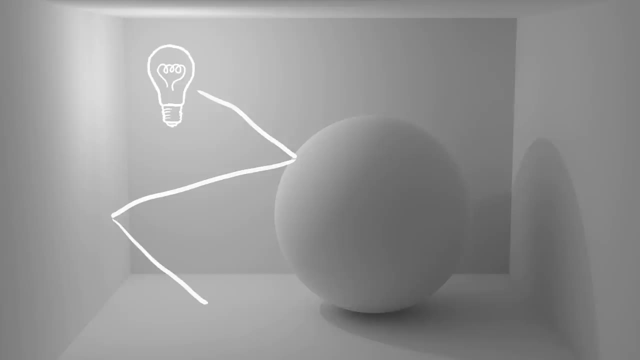 We can employ randomness. So whenever we hit a diffused surface, we simply pick randomly one of the infinitely many directions in which the light could be scattered. One randomly simulated light path on its own is not valuable, But if we generate many of these light paths, then we can simply simulate a diffused surface. 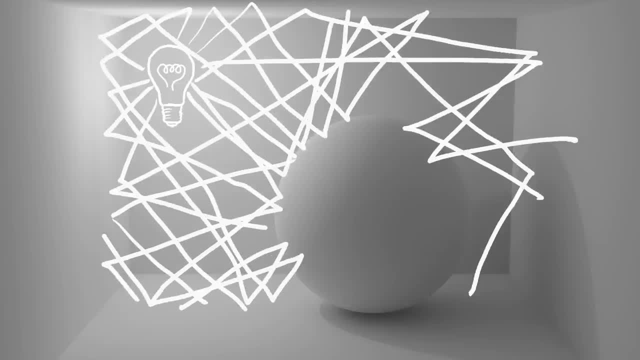 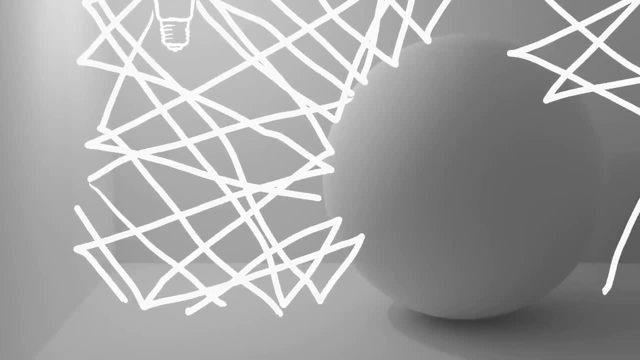 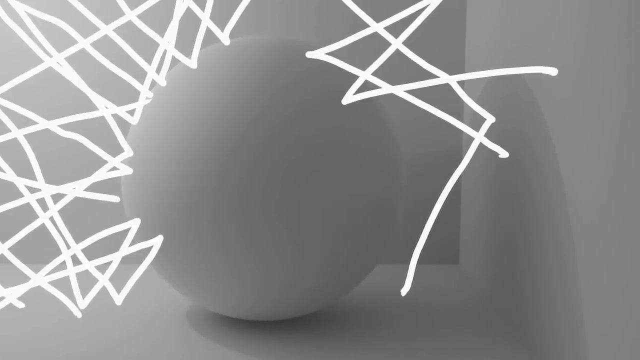 And then we have many sample paths that we get a good idea of the illumination of the scene. We will see areas that are hit by many of the randomly generated light rays and we'll see other areas that are hit only by few of the randomly generated rays. 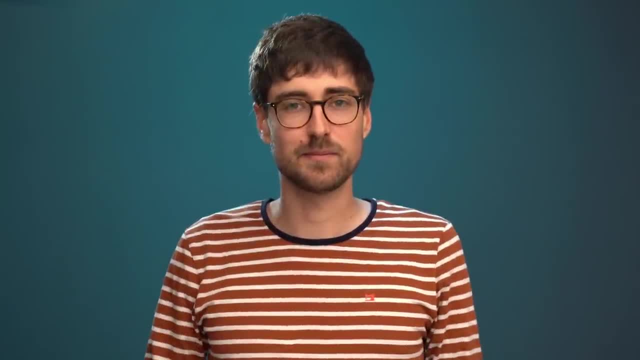 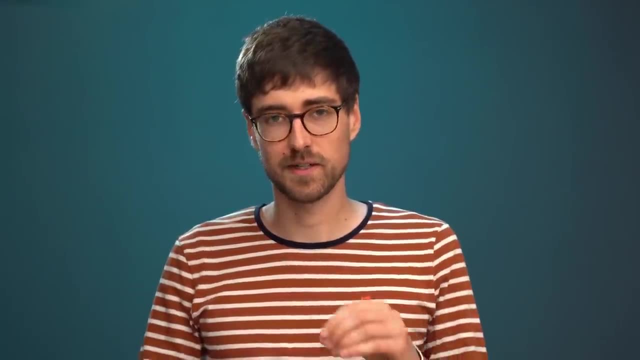 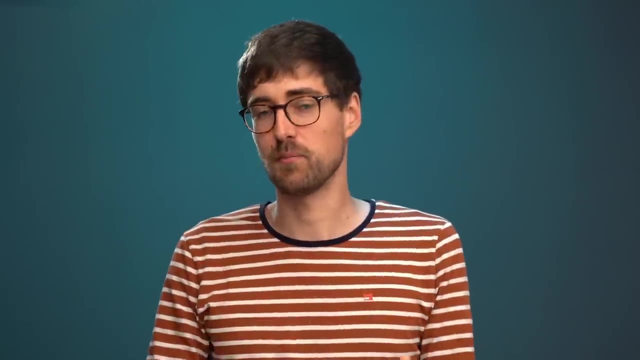 Darker areas. Actually, if you think about it, counting the number of randomly generated light rays hitting some area is really not that different from counting the number of random rays hitting randomly dropped marbles hitting some bowl And in this marble dropping attempt to determine pi, we saw that the result gets more accurate. 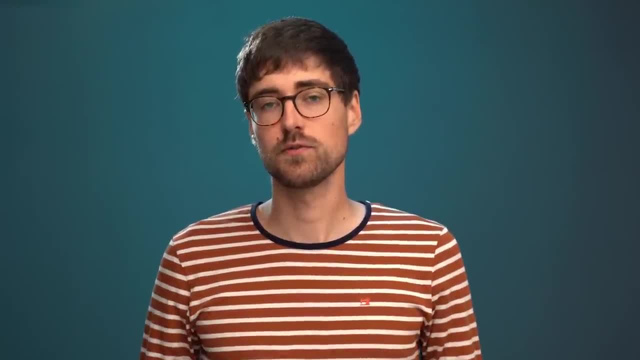 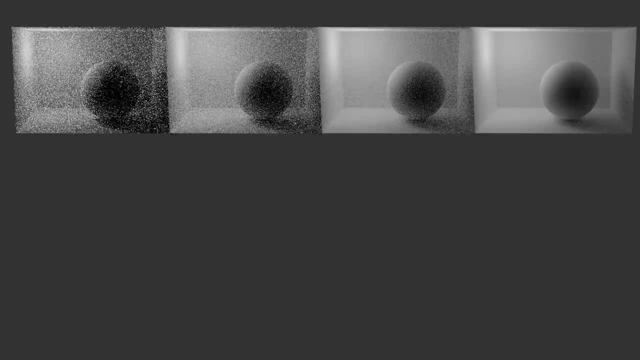 the more samples we take, And the same is also true for Monte Carlo path tracing. These four images show the same scene, rendered with a different number of randomly simulated light paths, And we can clearly see that with more sample paths, the result becomes more accurate. leading: 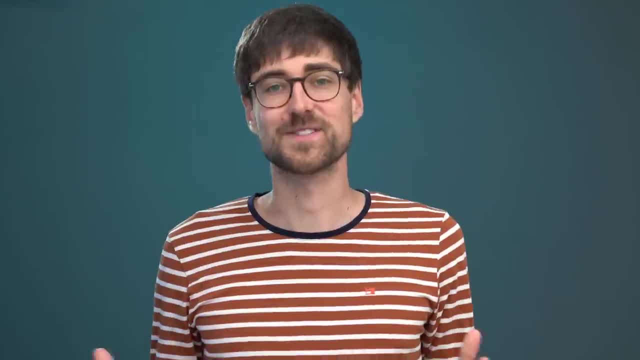 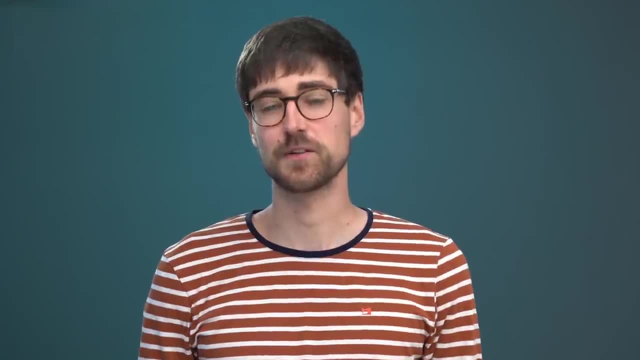 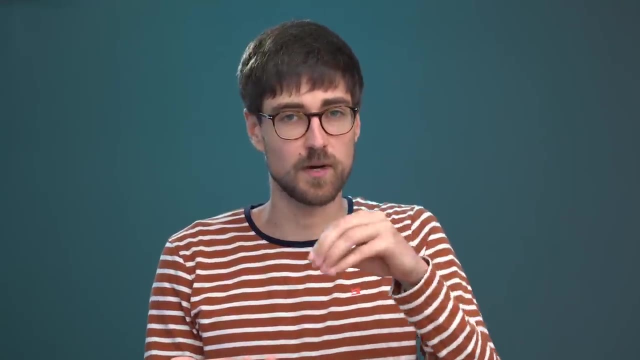 to a less noisy image. Okay, so let's wrap this up. A Monte Carlo simulation is a randomly evolving simulation, And in this video we have looked at two examples how such a randomly evolving simulation can be useful. We have determined pi by randomly dropping marbles into bowls.